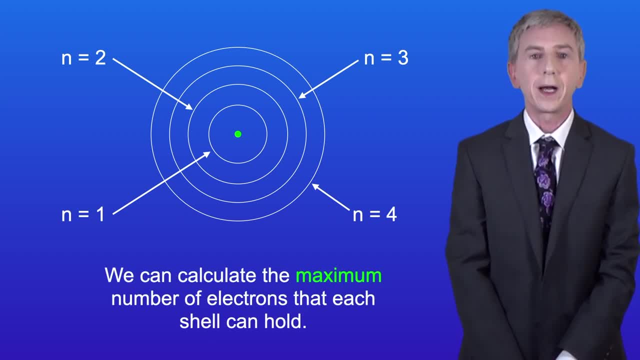 fourth is 4.. Now we can calculate the maximum number of electrons that each shell can hold, And to To do that we use this equation: The maximum number of electrons is 2 times n squared. Looking at the first shell, n equals 1.. 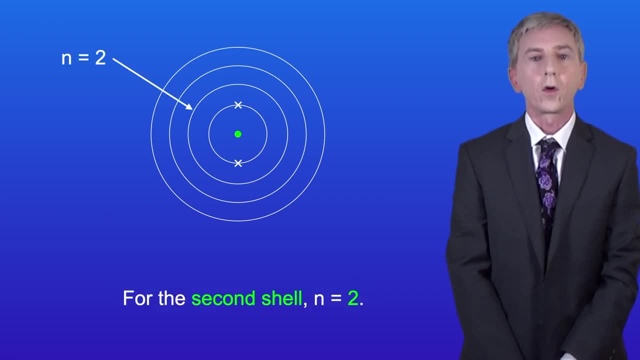 This gives us a maximum of 2 electrons in the first shell. For the second shell, n equals 2.. So this means that we've got a maximum of 8 electrons in the second shell. The third shell can hold a maximum of 18 electrons and the fourth shell can hold a maximum of. 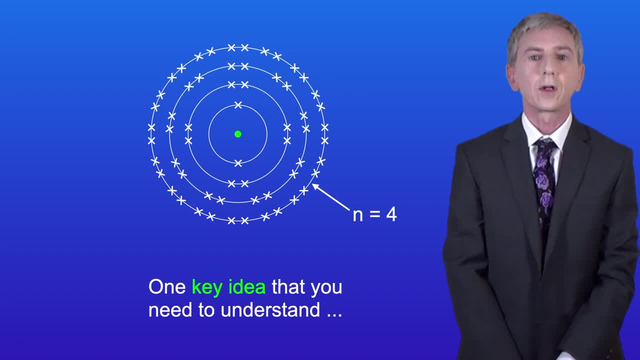 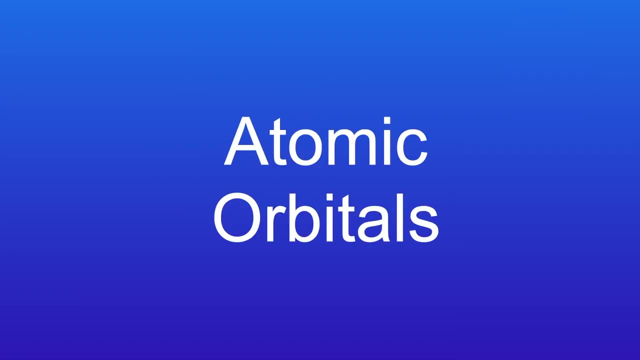 32.. OK now, one key idea you need to understand is that the electrons in a shell are found in regions called atomic orbitals, and we're going to look at those next. OK, I'm showing you the definition of an atomic orbital here. 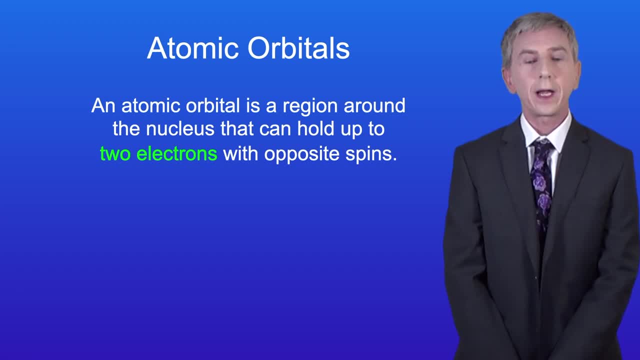 An atomic orbital is a region around the nucleus that can hold up to 2 electrons with opposite spins. Now for chemistry, A level. you're not required to know what spin is. however, you do need to know that electrons can either have an up spin or a down spin. 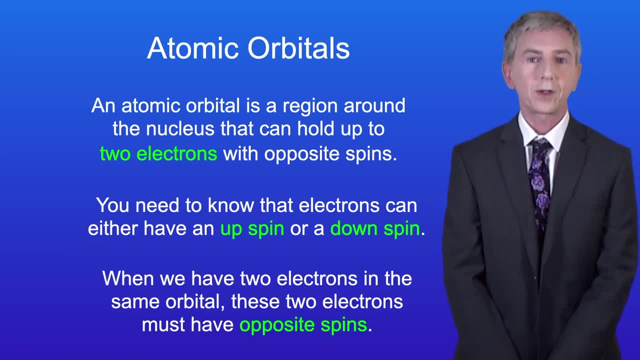 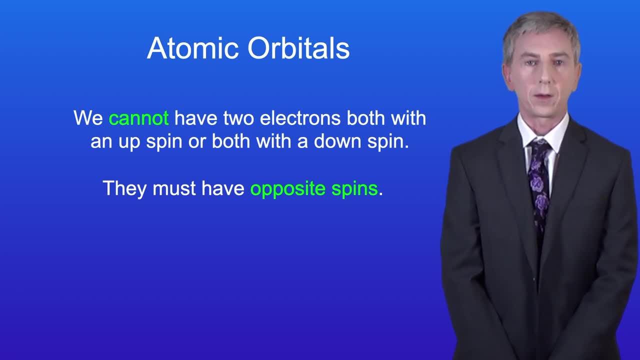 Now, when we have 2 electrons in the same orbital, these 2 electrons must have opposite spins. We cannot have 2 electrons both with an up spin or both with a down spin. They must have opposite spins. Now, at GCSE we consider an electron to be a particle. however, at A level, an electron 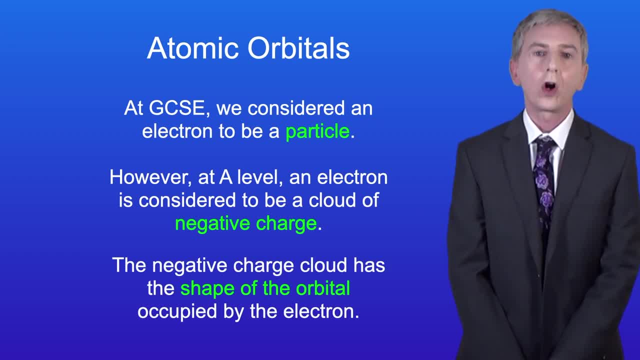 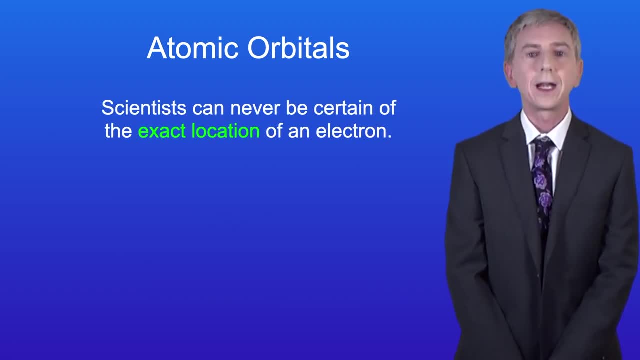 is considered to be a cloud of negative charge, and the negative charge cloud has the shape of the orbital occupied by the electron. Now, one idea you need to be aware of is that scientists can never be certain of the exact location of an electron. The atomic orbital shows us a 95% probability of where an electron will exist. 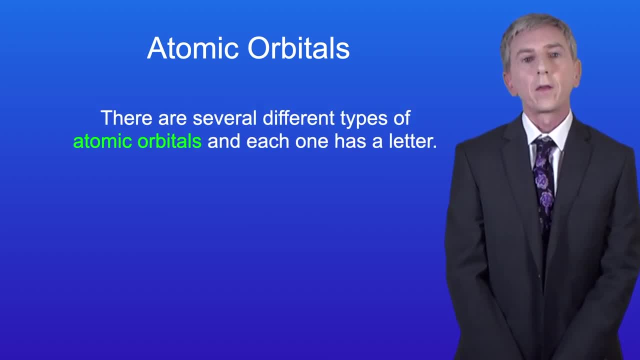 So we need to be aware of that. OK, now let's look at an electron. There are several different types of atomic orbitals, and each one has a letter. These are S, P, D and F. We're going to start by looking at the S and the P orbitals. 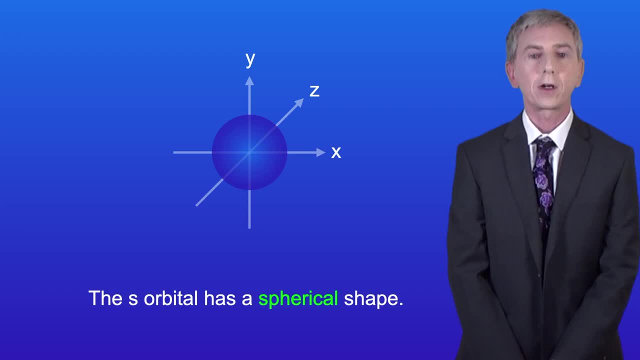 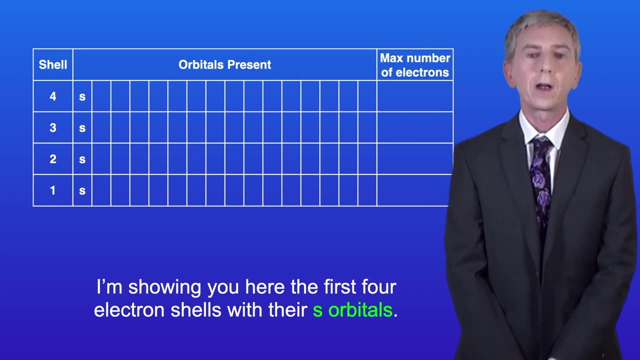 I'm showing you the S orbital here and, as you can see, the S orbital has a spherical shape. Every electron shell contains a single S orbital. So I'm showing you here the first 4 electron shells with their S orbitals. OK, let's take a look now at the P orbitals.